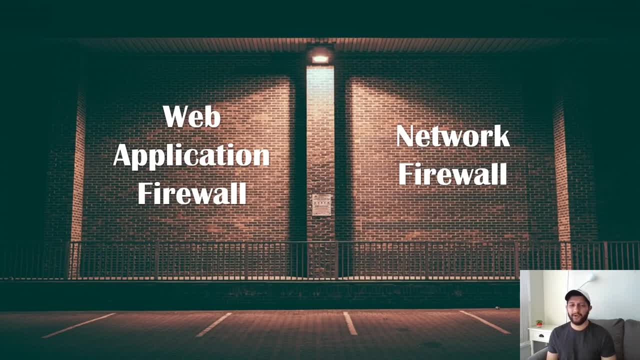 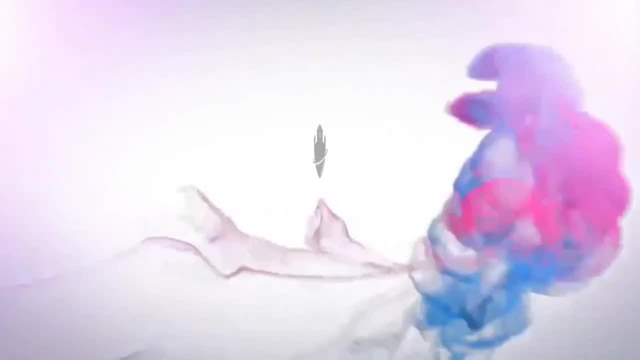 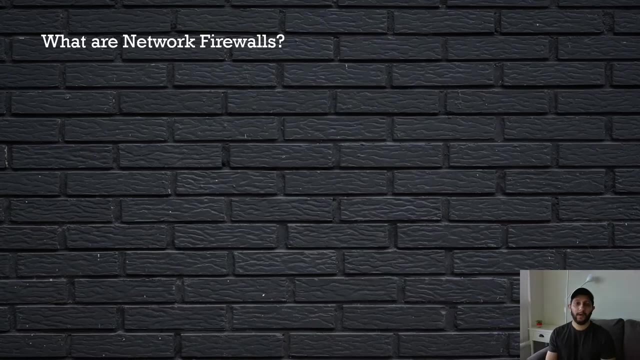 on layer 7 of the OSI layer. the other one works on layer 3 and layer 4.. So, without further ado, let's get into the video right after this short intro. So what are network firewalls? Well, network firewalls are nothing but security devices. 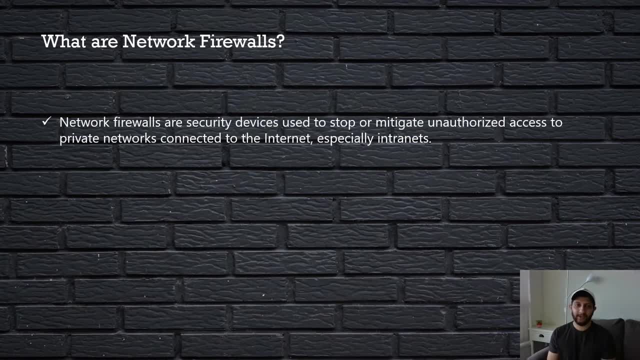 that are used to stop and mitigate unauthorized access to your private network, which are exposed to the internet. Now how do we do that? We write policies on that firewall. These policies are designed in such a way as in when an unauthorized traffic tries to enter your corporate network. 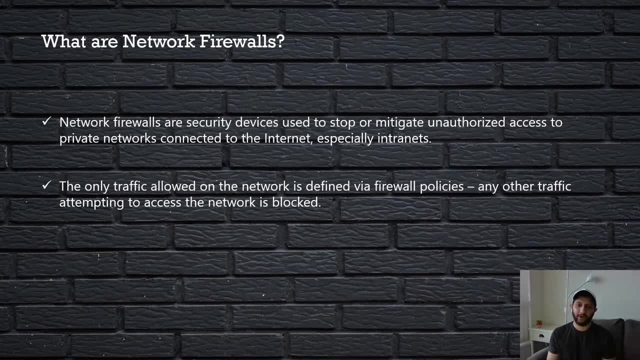 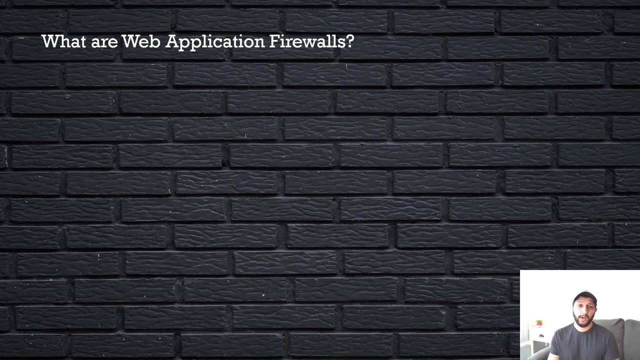 that policies get triggered and then block the traffic completely. Now where do we place that firewall? It is usually placed on the perimeter end, that is, the front line between the internet and the internal network. So what are web application firewalls? A WAF helps protect. 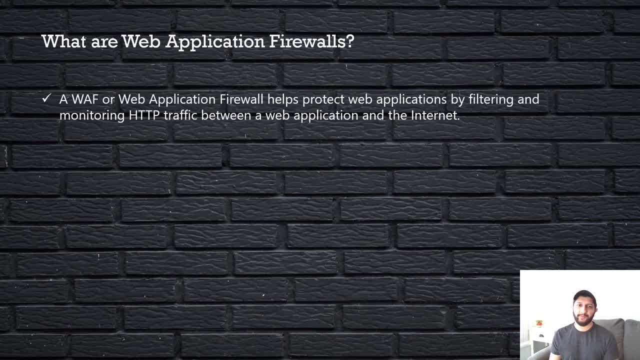 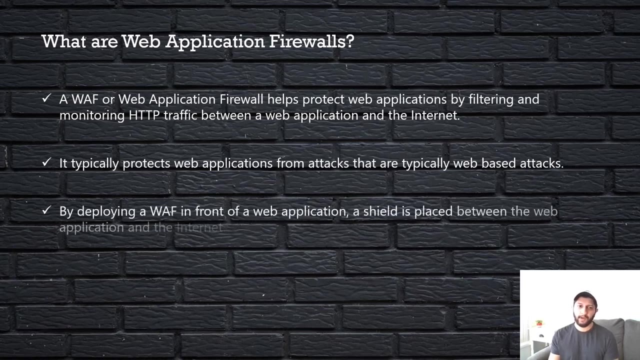 web applications by filtering and monitoring http traffic between a web application and the internet. What does it protect from? It usually protects from the web-based attacks that enter the network via layer 7 of the OSI layer, that is, the application layer. Now, how does it protect? It usually behaves. 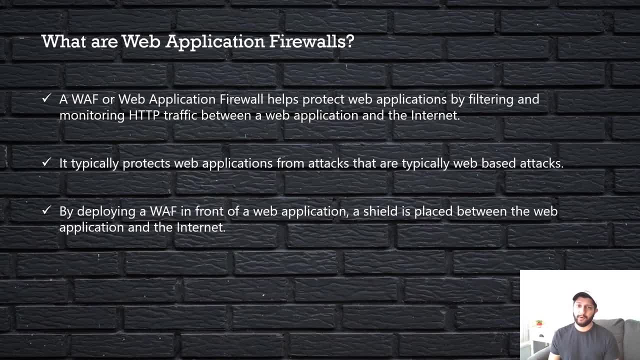 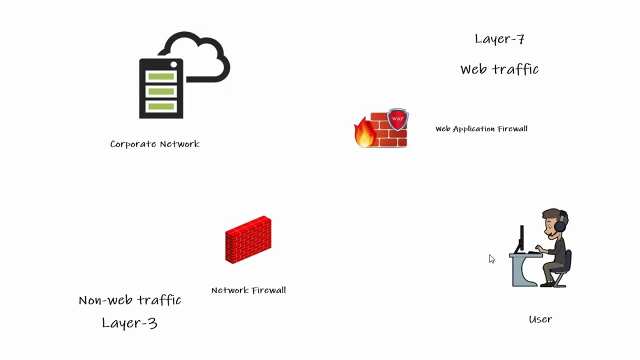 or you know, believes as a shield over and above the next-gen firewall, that's the network firewall, just so that the layer 7 and the layer 3- both layers are protected, All right. so let's understand this concept graphically, with some features around. So say you're a user on the internet trying to access a few web applications. 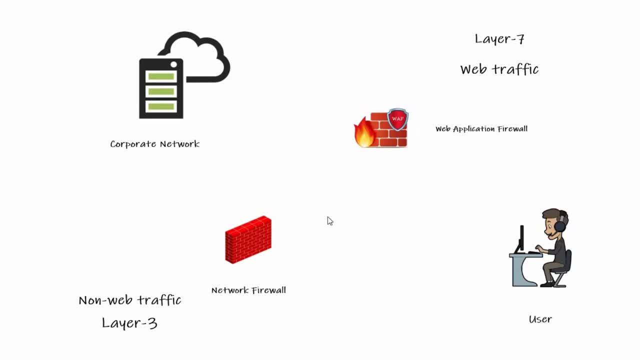 on the corporate network. Now the corporate network is behind the WAF and the network firewall, So your request will go to the WAF, The WAF will send it to the network firewall and then it will send the request to the corporate network and then the corporate network will. 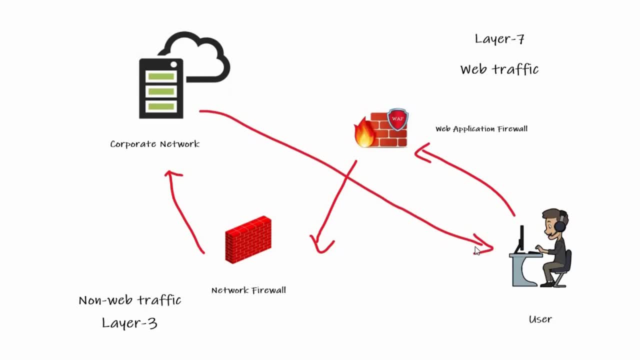 send you the request with some access permissions accepted for the web application. Now, had we not had the WAF in place, the request would directly go to the network firewall. The network firewall will forward it to a corporate network. Now here's the catch: The network firewall.